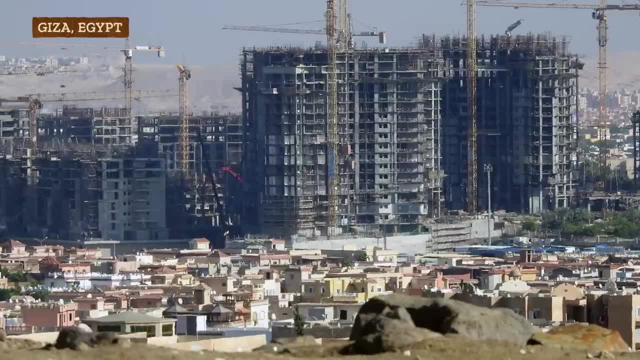 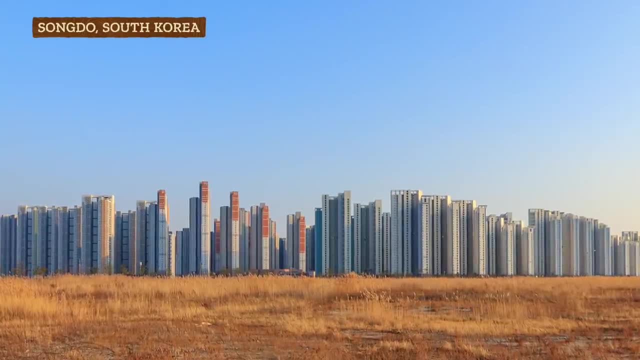 hall to our houses reflect our cultural traits, But they're also a product of our economic and political relationships, And even if we build a city from scratch, it tends to reproduce the social relationships of our time. Why and how this happens is part of the focus of urban geography which we've been studying. 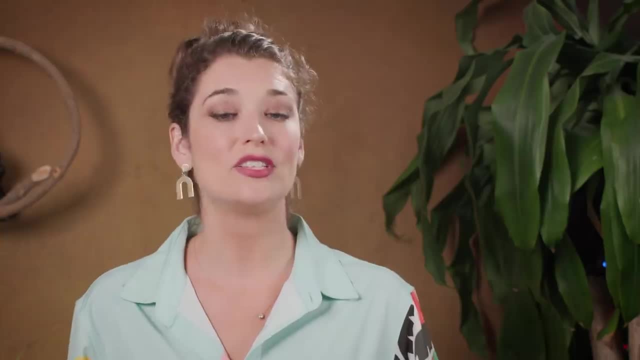 for two episodes now. As urban geographers, we try to understand the pattern of urban geography and how it's important to us. As urban geographers, we try to understand the pattern of urban geography and how it's important to us. 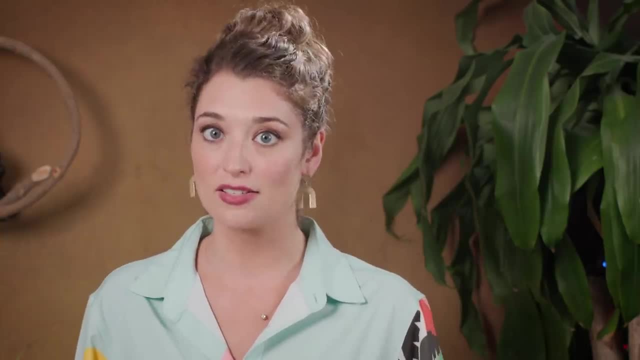 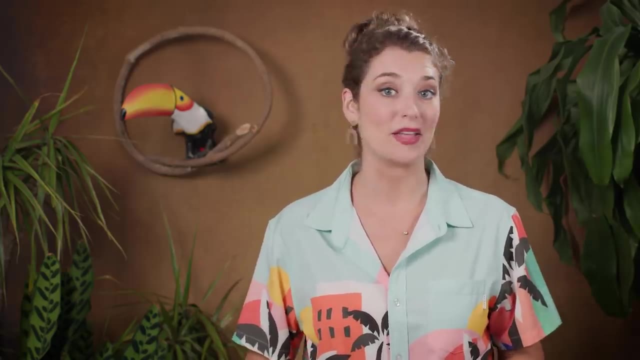 We try to understand the patterns behind where people settle and how land is used in urban areas and why those patterns change over time. To do that, urban geographers use models and economic processes to predict the future and try to explain the present, Like what cities will look like in the future or how a city 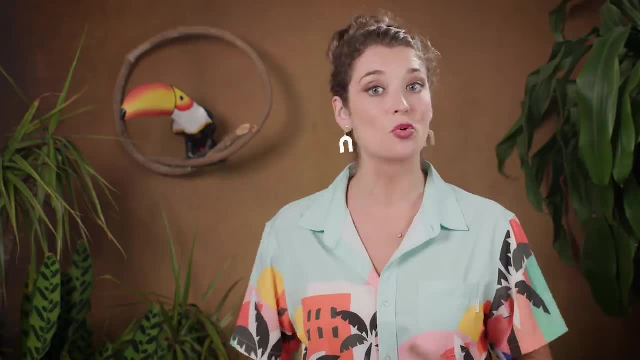 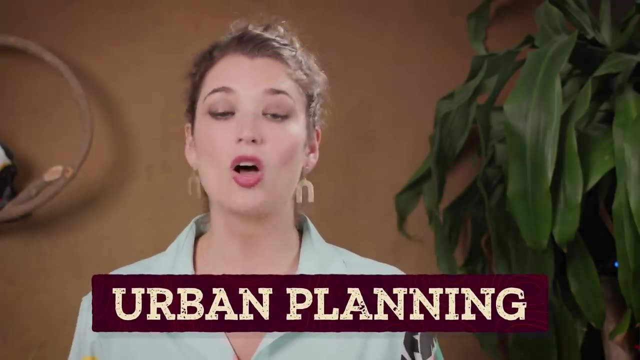 developed and how the work of past urban planners and geographers either helps or prevents people from accessing good homes or jobs. And within urban geography, we can get even more applied with urban planning, which is all about the design and regulation of space within urban areas. 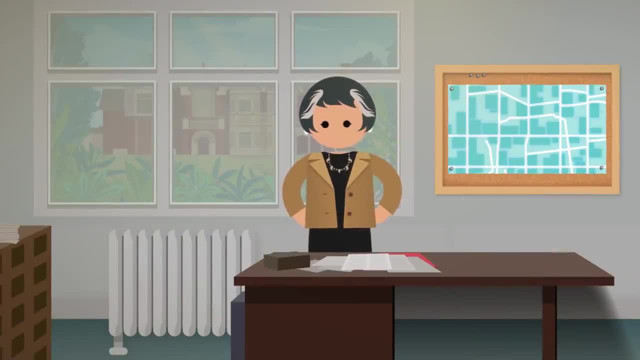 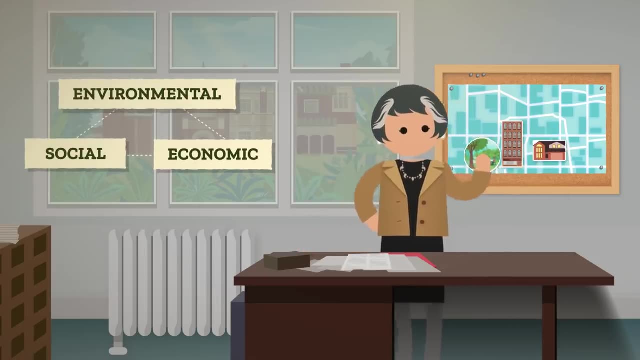 Urban planners work for governments and non-governmental organizations like land conservation groups. They weave together the economic, social and environmental goals of the region with the intent of creating zones of work, play and living that will benefit the region. As urban planners, we have a tremendous influence on people's lives. 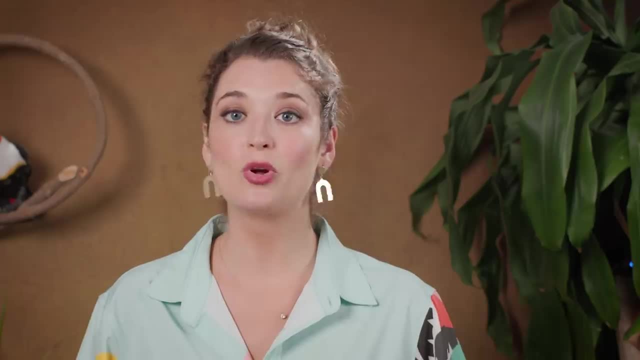 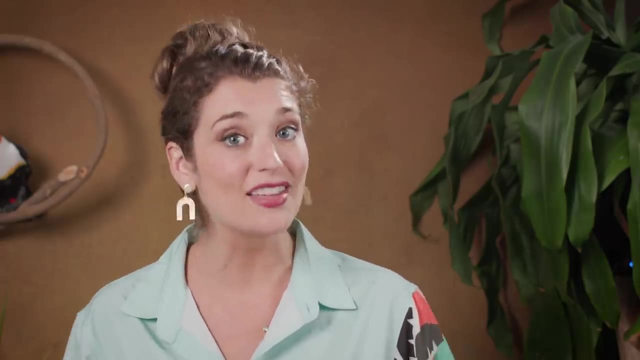 And there's a lot to consider. So for the next three episodes we'll explore different types of planning and how we think about space and understand the relationships that guide where and how humans build cities and everything in and around them. Historically, there have been lots of different ways of planning. 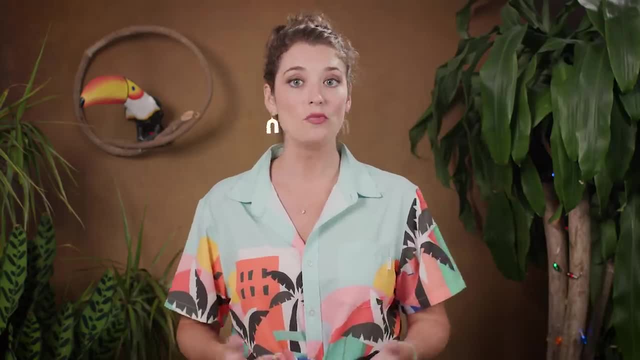 There have been lots of different ways of planning. There have been lots of different ways of planning. There have been lots of different ways to plan cities, And different cultures have their own patterns of urban development Or how cities grow and change. For example, there's the Latin American model. 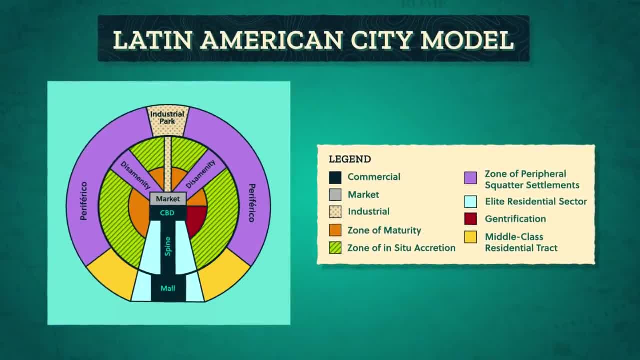 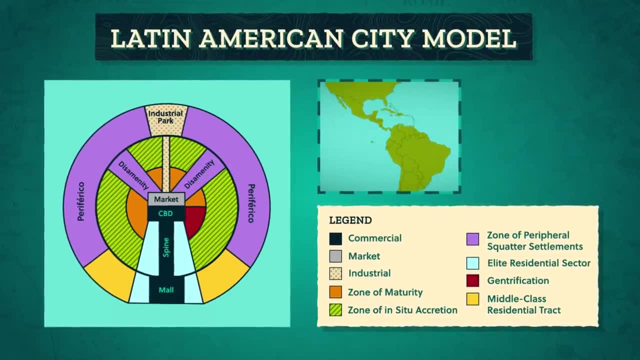 This model describes the types of cities mostly Spanish colonizers designed as they built up cities throughout what's now Central America and much of the American West and Southwest, often on the same land as indigenous cities they had destroyed, And the way any society designs their towns and cities, whether centuries ago or today. 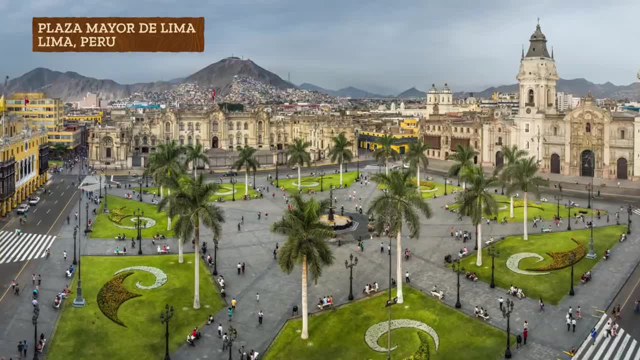 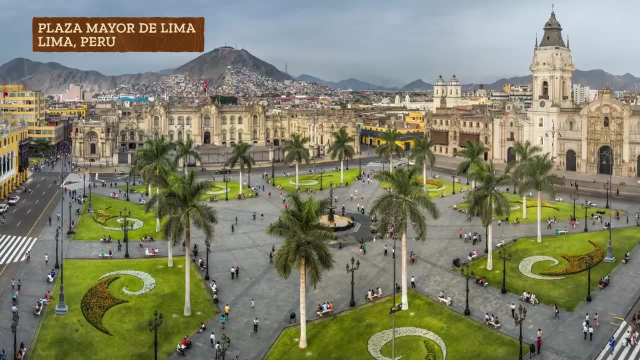 will give us clues about the goals of the leaders of that society. In the cities of Latin America, colonial priorities are built into the city, like how they include a plaza with cathedrals and space for markets and a grid of streets, like the cities in Europe. 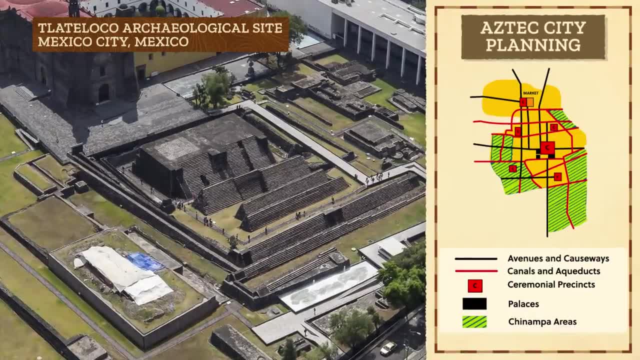 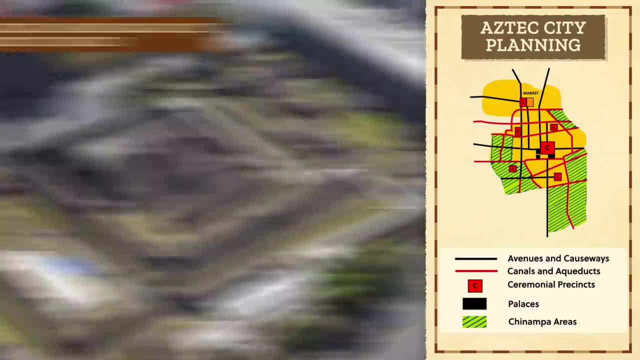 For indigenous peoples like the Aztecs. the central plaza was an element that was also used in planning and urban design, with prominent buildings, a palace, a temple and a place for ball courts and sacred areas, And in pre-colonial times, the way housing was located, both planned and unplanned, varied. 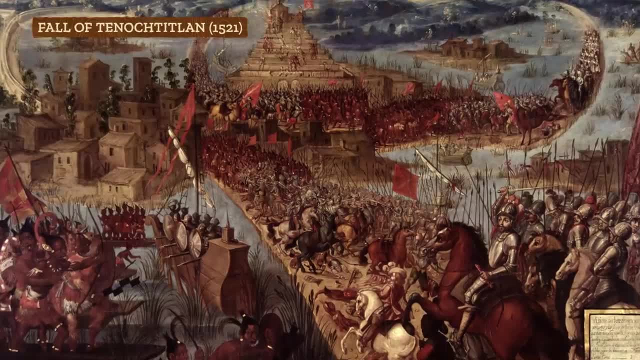 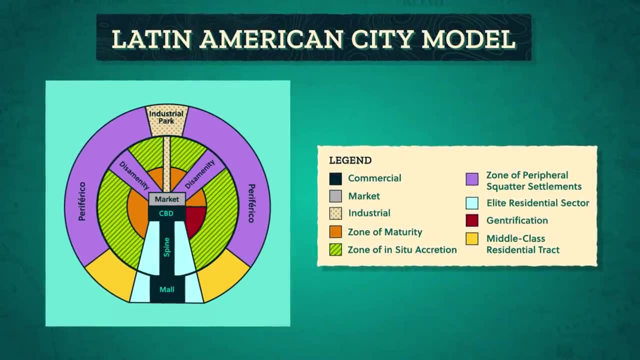 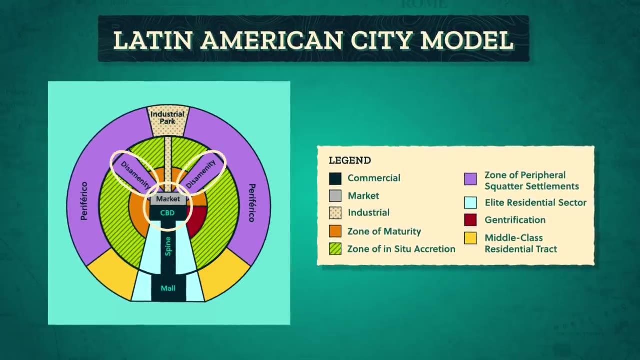 across Latin America, even within similar empires. But that shifted with the arrival of colonizers. In the Latin American model, showing wealth and social status through housing arrangements became a common design. Housing for the wealthy developed around that central market And radiating out from the central market to the periphery are zones of disamenity. 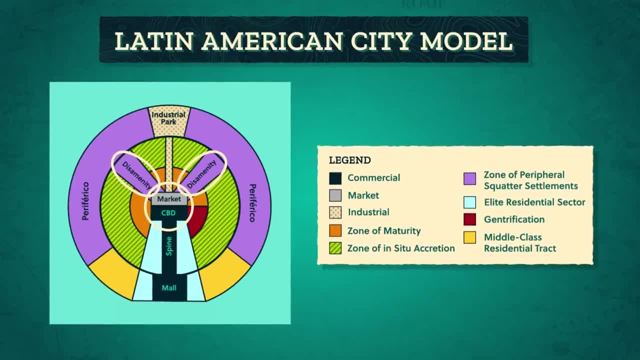 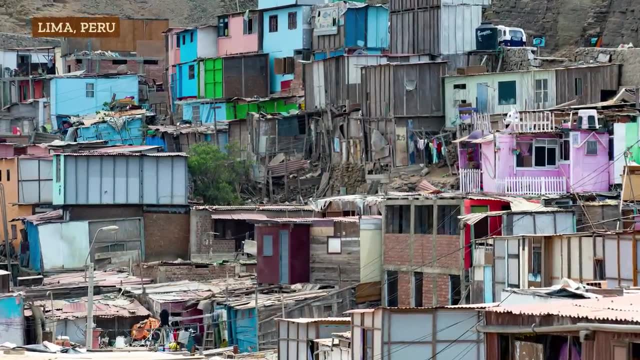 which are corridors of squatter settlements made up of thousands of people in the city who can't afford a house or land, but who still need a place to live. Squatters tend to build their houses out of whatever materials are available, And this is a highly precarious living arrangement. 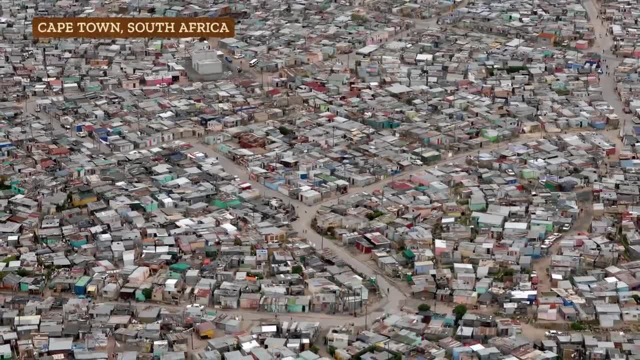 And even though it's a common type of neighborhood in low-income areas in many cities around the world, the lack of legal access to housing is a common problem, And the lack of legal rights to the home in which they live makes it easy to displace. 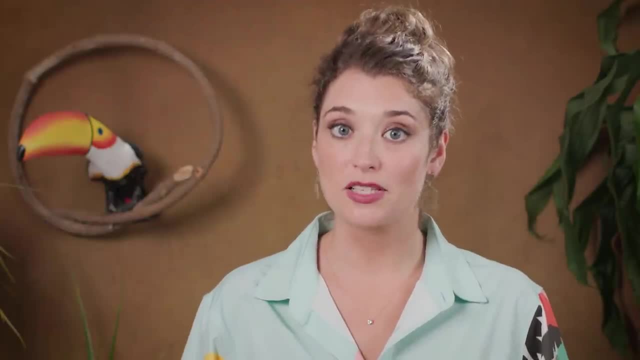 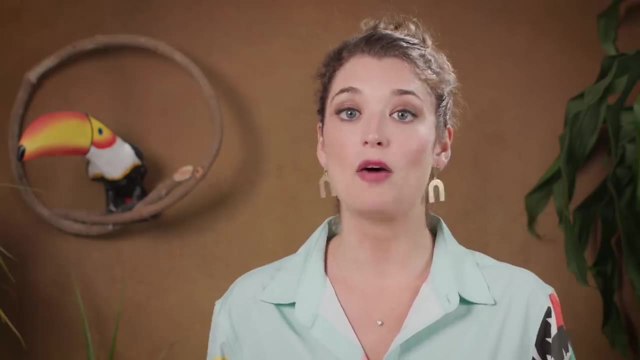 these communities. So how a city is structured influences how it develops and tells us about the things the people living in it value. It can also tell us how we imagine our city in the future- things like how many people might live in the city or what types of industry might be there. 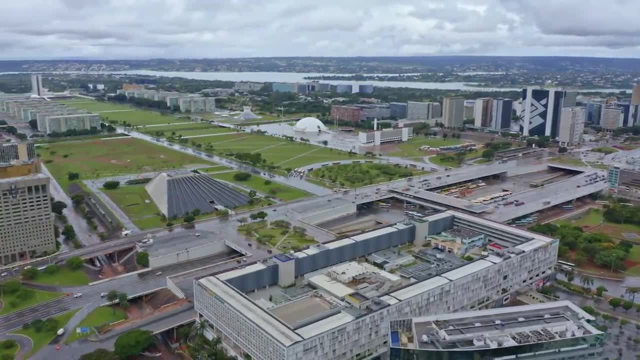 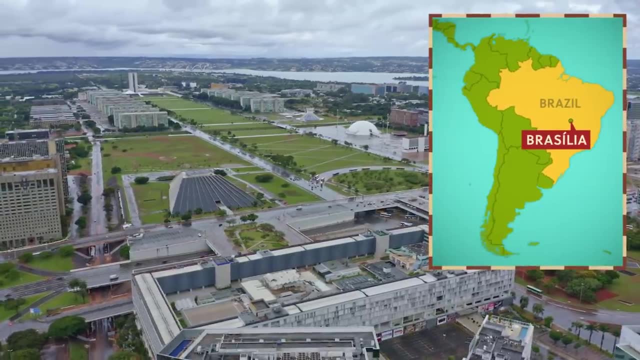 Like in the 20th century, city planning in Latin America tried to fix or prevent these zones of disamenity from happening, while also creating regions that thrive economically and socially. Take, for example, Brasilia, the capital of what we call Brazil. 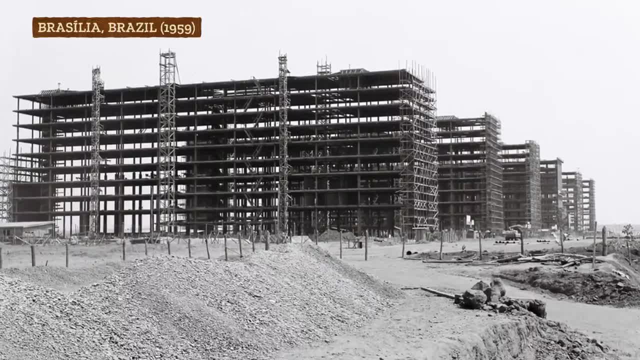 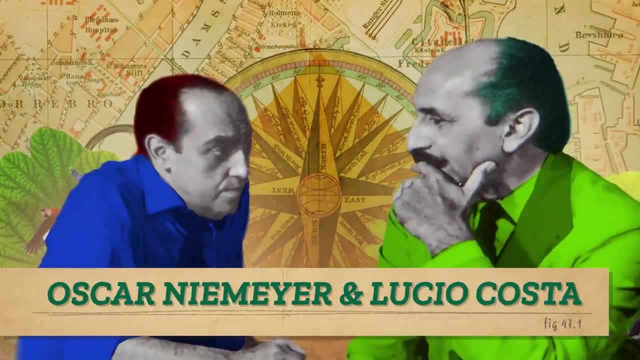 The area wasn't even a city. It wasn't even a city by the early 1950s, when Brazilian leaders decided that by 1960 it would finally be the new site of the nation's capital. Urban planner Lúcio Costa won the design competition and invited his friend and architect. 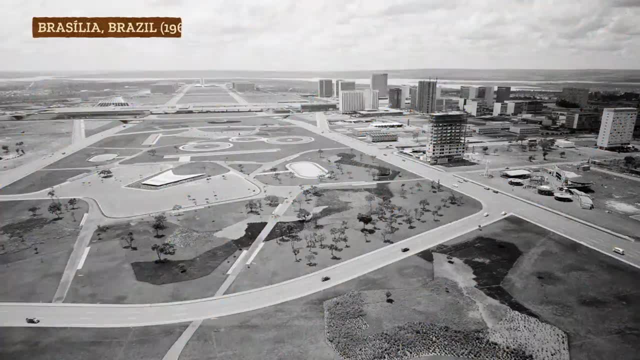 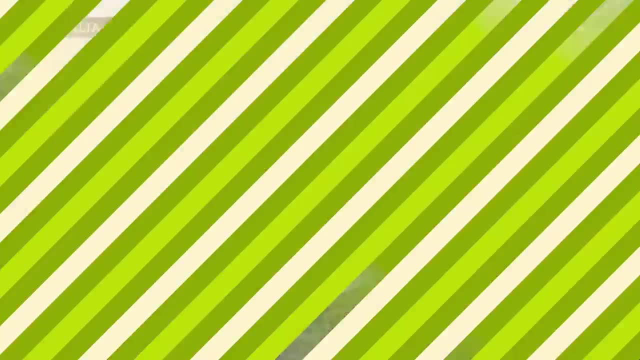 Oscar Niemeyer to make his vision of a modern city a reality. They wanted to create something innovative that would both open development to the interior of Brazil and be an urban place without the poverty of older colonial cities, Unlike the traditional Latin American model, Brasilia was designed to look like a bird. 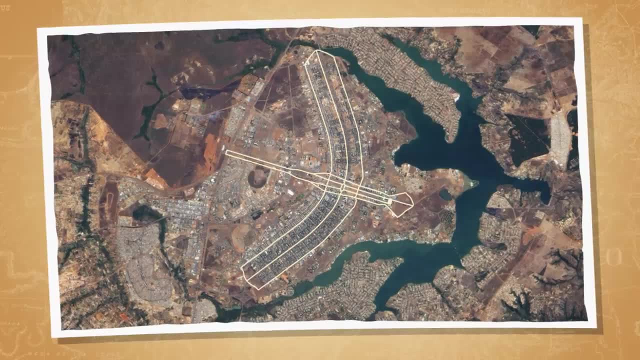 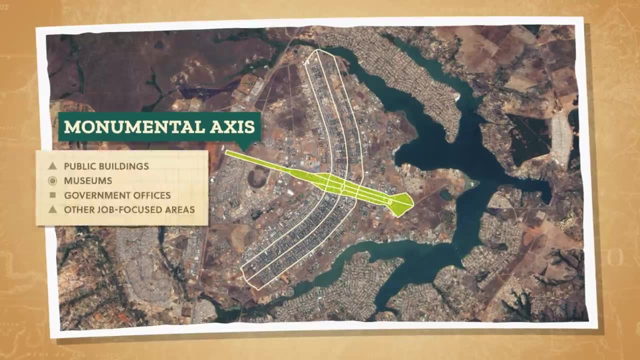 or airplane flying off into the future, And it's much farther inland than other major Brazilian cities. Overall, the original city was made up of one monumental axis, or the body of the bird, which contained the public buildings, museums, government offices and other job-focused 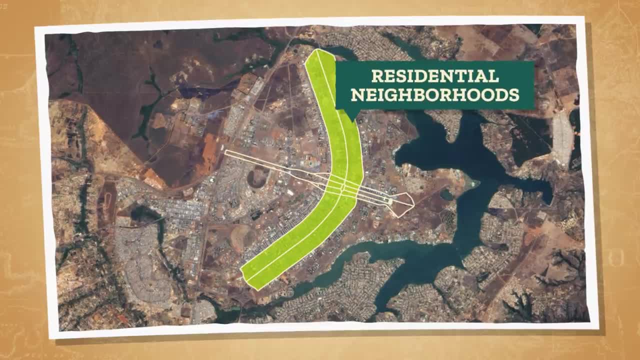 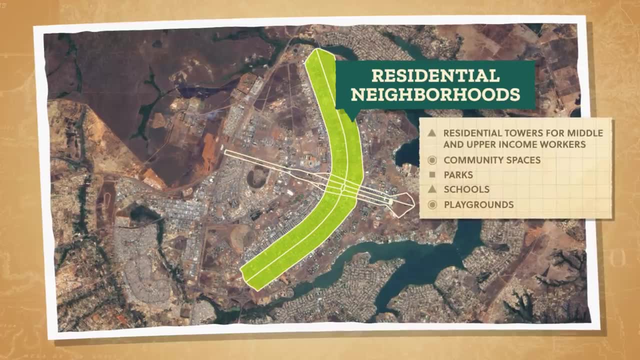 areas And the two wings contained the residential neighborhoods. These superquadras contained residential towers for middle and upper income workers from the monumental axis, as well as community spaces, parks, schools, playgrounds and, in theory, everything a community would need. 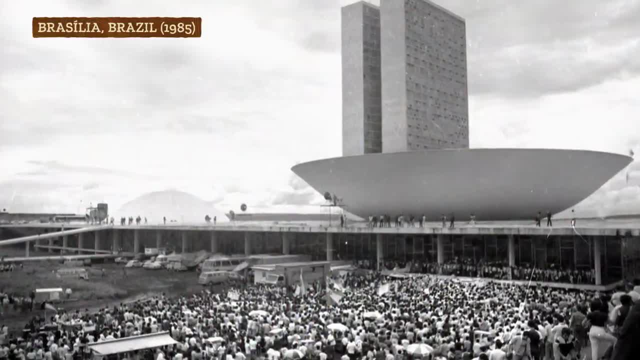 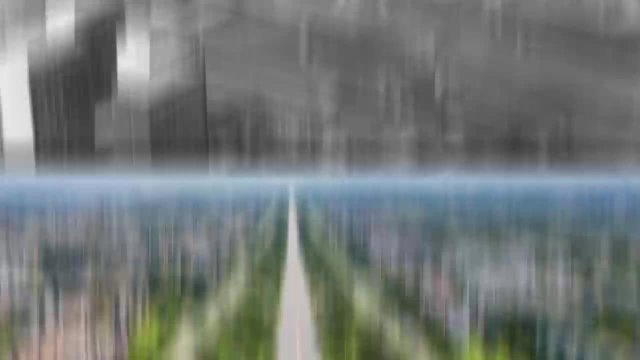 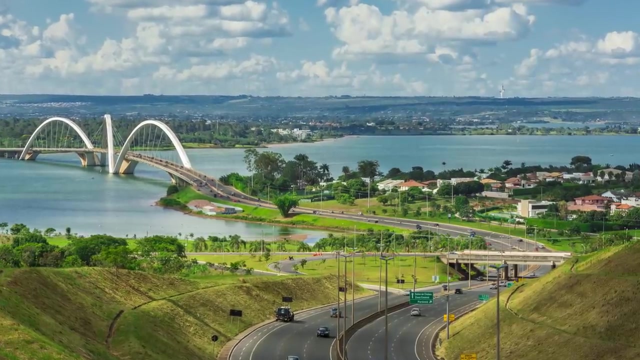 Brasilia was designed based on a vision of the future from the 1950s and it doesn't match how people want to live their lives today, in 2022.. The city was designed to rely on cars and even to try and separate where people worked. 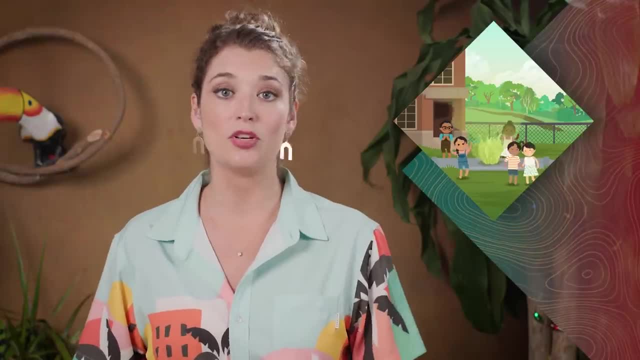 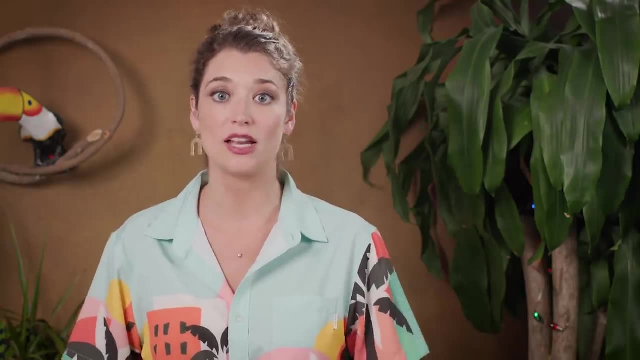 and lived, And while most people agree that not all mixing is good, like we don't want toxic industries spewing chemicals near homes and schools, robust communities do have some level of mixing between commercial and residential, like shops, office work and houses. Being able to work and live close together is important for keeping transportation costs low and maximizing how many services a person can easily reach from their home, But the relationships that form in a city inevitably bubble up and imprint themselves on the landscape anyway. Brasilia was designed for 500,000 people, but by 2020 there were over 4.6 million people. 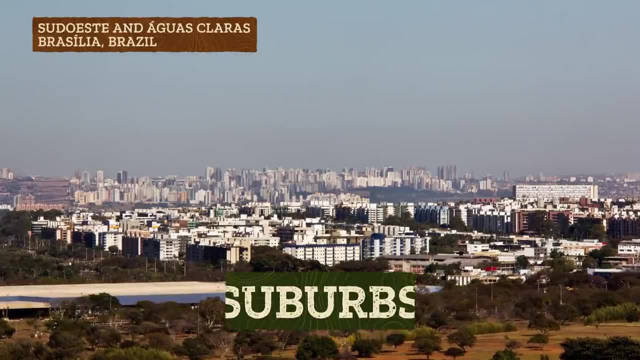 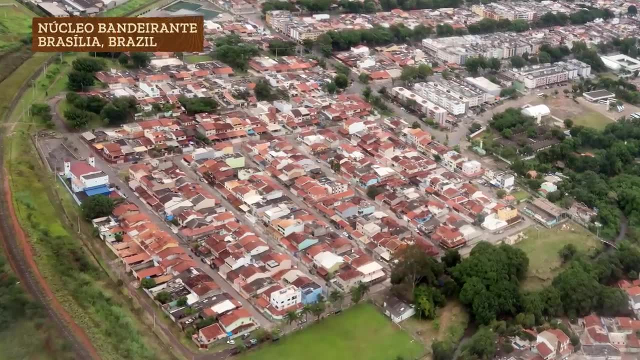 living there. All those people couldn't all fit in the original wings, so suburbs or low-density, car-dependent areas outside the main city developed In Brasilia. they're called satellites and they grew organically and do not match the aesthetic of the rest of the city. 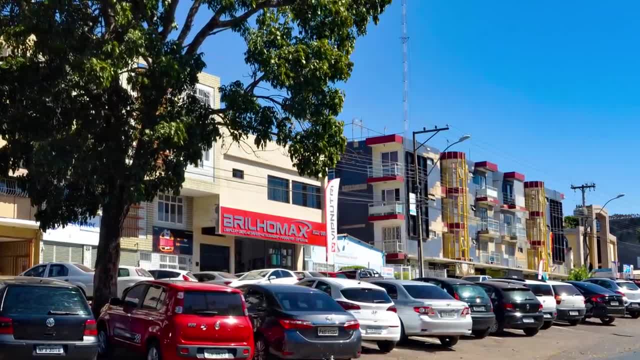 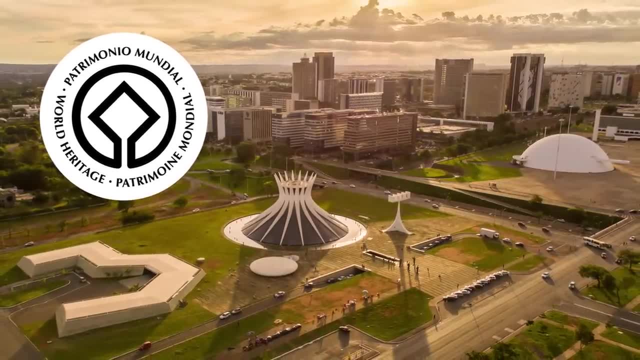 They're vibrant, with people living and working in the same areas, and contain the messiness of uneven access to resources and jobs. Today, Brasilia is a UNESCO World Heritage Site because of its ambitious and unique urban design. It's an example of how we can plan something on paper, but a city is a space that encapsulates. 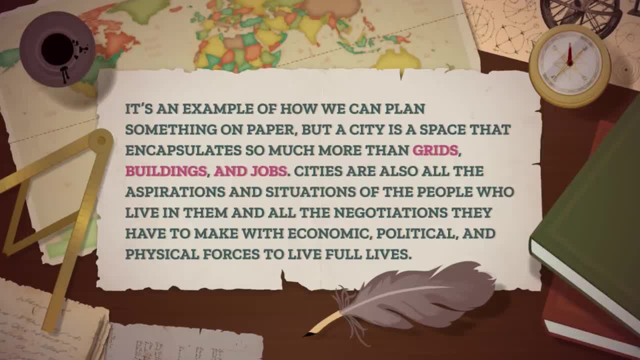 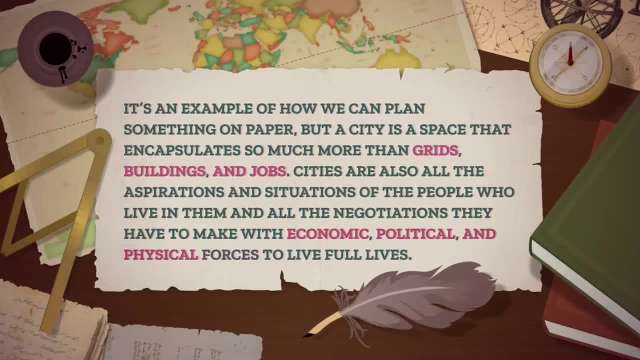 so much more than grids, buildings and jobs. Cities are also all the aspirations and standards And situations of the people who live in them and all the negotiations they have to make with economic, political and physical forces to live full lives. 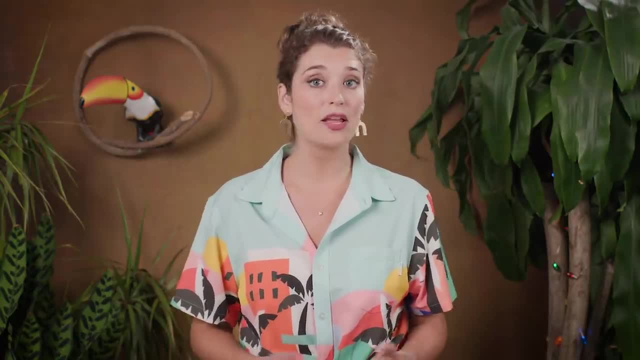 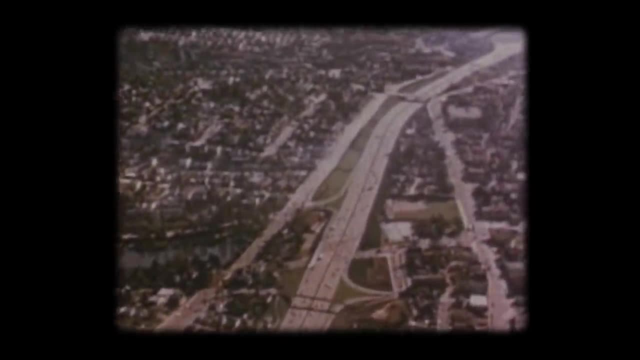 But not everyone is allowed to live full lives or build community, And urban planning can play a role in that, For instance, in urban sprawl and white flight in the United States, which was the progressive movement of white people farther and farther from the center as they gained wealth and as minority populations moved into the city, Urban planning also helped to facilitate that movement. In the 1960s there was an infusion of investment in the US highway system and being able to get places quickly helped shift the location of entertainment and shopping from town centers. 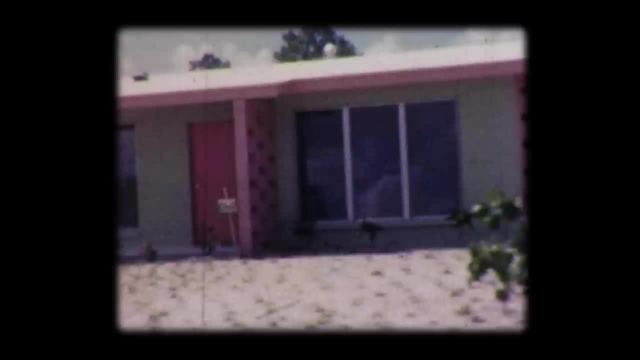 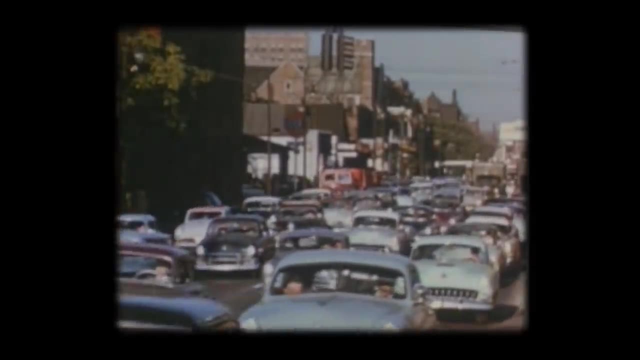 to stand-alone complexes and edge cities. There were also incentives like affordable land to build new homes and low-interest home loans to World War II military veterans. All that, coupled with low fuel costs and other lingering effects from World War II, made it possible for those in the middle and upper economic classes to leave cities and move. 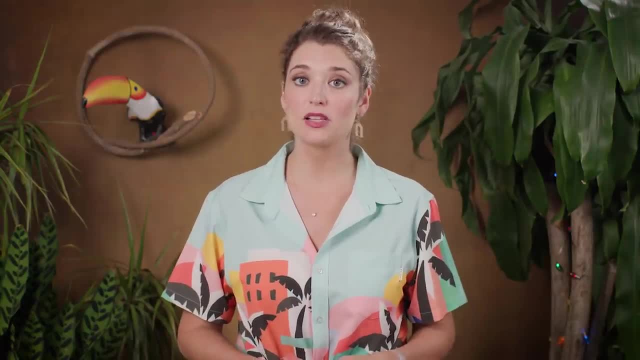 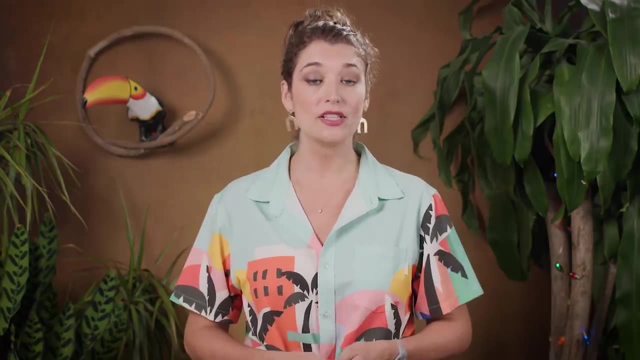 out to the suburbs. Well, it made it possible for some people Because there were also forces working hard to keep minority Americans from owning land and houses, Especially Black and Asian Americans. For instance, if we go back to the 1930s, some forces to prevent people from owning 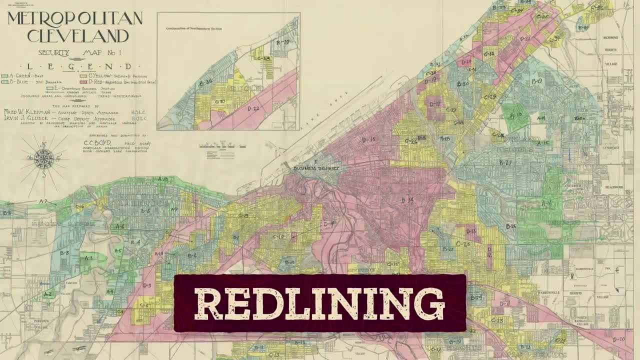 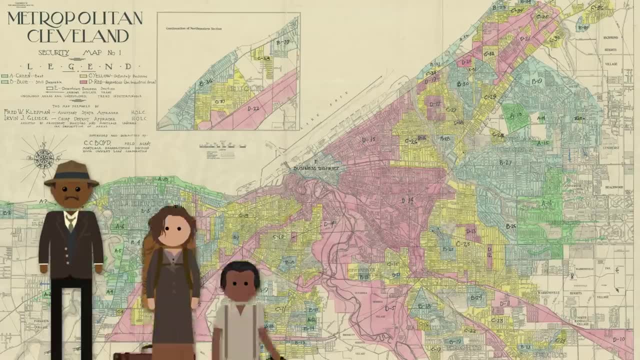 land were already in effect. Redlining is when urban maps were color-coded to indicate which neighborhoods were considered high risk to lend money to The credit of people in Black neighborhoods, followed by those of recent immigrants, was rated the highest risk level and outlined in red. 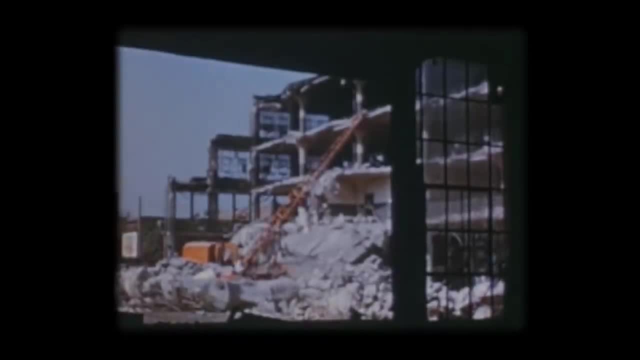 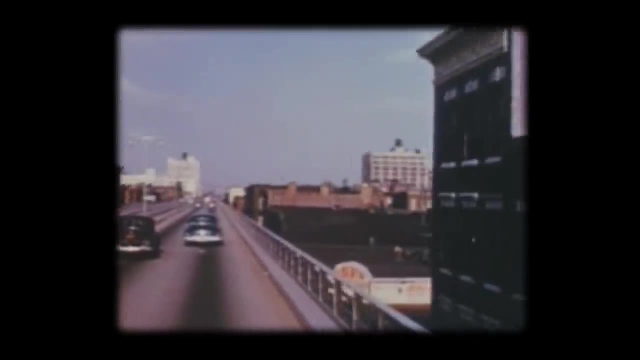 This made home ownership and land ownership very difficult, And it got even harder in the 1950s. After almost 20 years of planning and discussion, the auto industry and highway engineers were able to build a complex interstate system from coast to coast, one that cut right through. 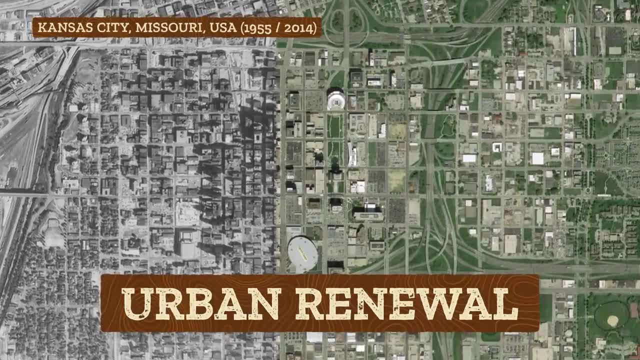 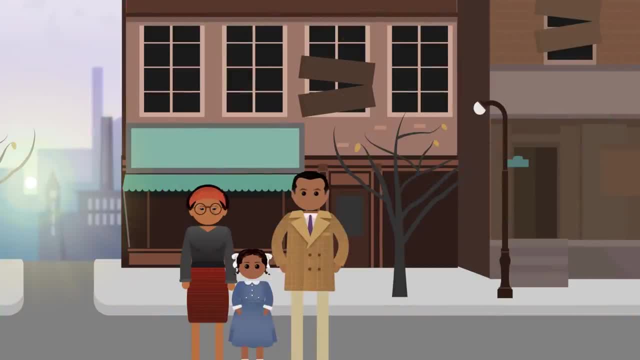 many cities, This paved the way literally for urban renewal, which was a process in cities that allowed them to clear away areas deemed as blighted to allow for new construction. Overwhelmingly, those freeways went through historically Black neighborhoods And the houses that were removed did go through the process of eminent domain, where a landowner must be compensated for property taken for public use, But because many of the residents were not, and effectively could not be, landowners, they received minimal compensation, if any. The properties were also undervalued, so anyone who did receive compensation rarely got enough. 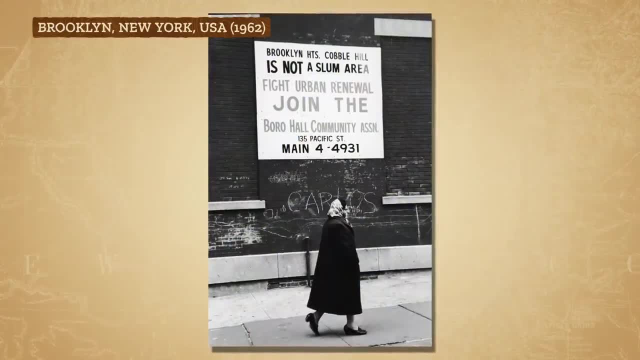 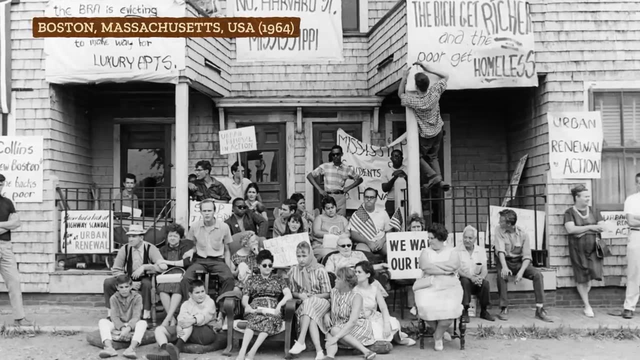 to move to a similar neighborhood elsewhere. So we have to remember that urban planning is part of larger social systems and can be abused by those in power. In the US, the freeways and easy movement that allowed suburbs to thrive also involves a history of redlining and urban renewal that allowed some neighborhoods to wither. 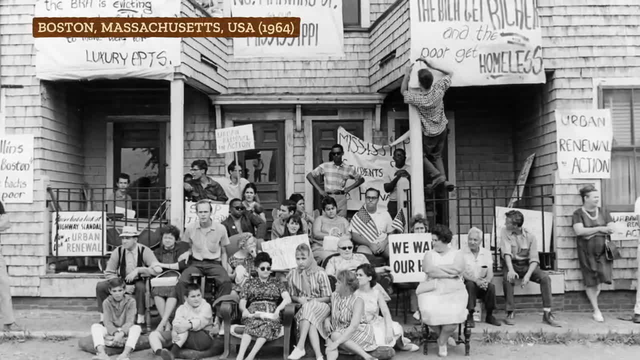 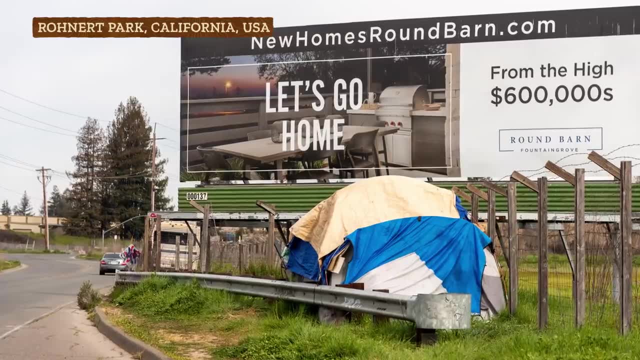 Other places. they created segregated neighborhoods with limited access to financial resources. Legally, redlining may have ended, But that's not all. In the US there's a lot of redlining, But unfair housing and real estate access are still problems. many Black people and other. 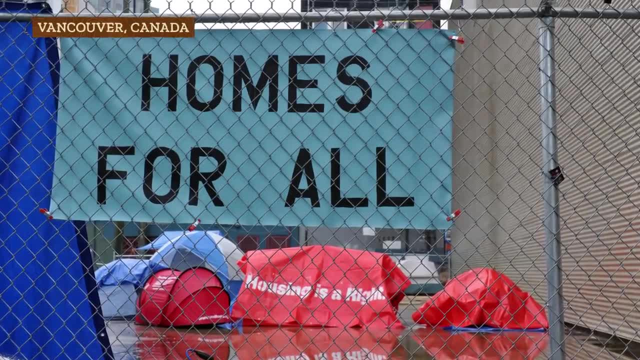 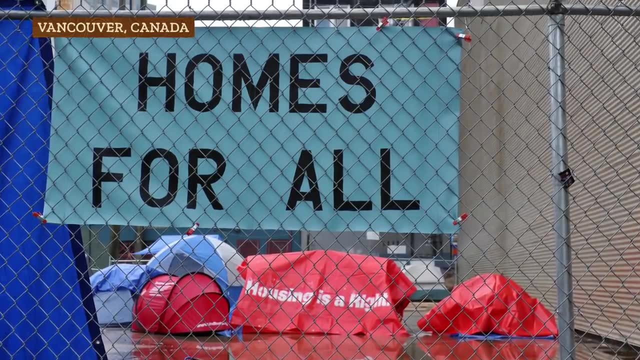 minorities face. So any efforts to build poverty-free cities in the future or any efforts to eradicate the urban poverty that already exists must intentionally address the structural disadvantages built into the way our cities and communities are designed, Whether it's social status in colonial cities in Latin America, wealth and community, and 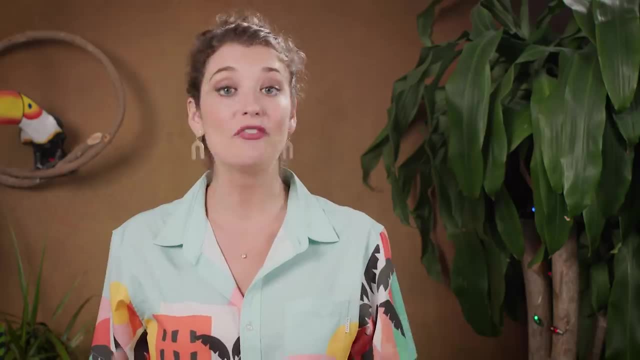 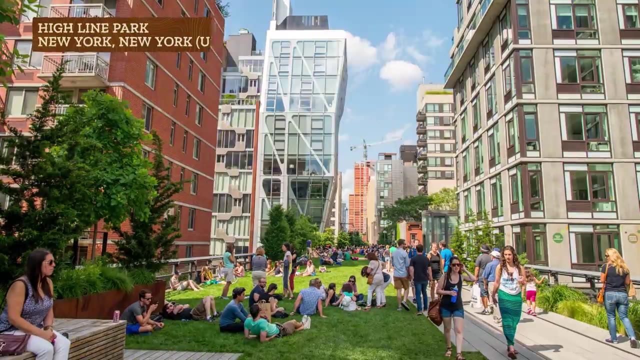 innovative design in Brazil or race in North America. every choice that's made about where to allow different types of land use reflects the relationships and values that the city has to make in order to make those decisions. While urban planners understand the social and economic mechanisms that create vibrant